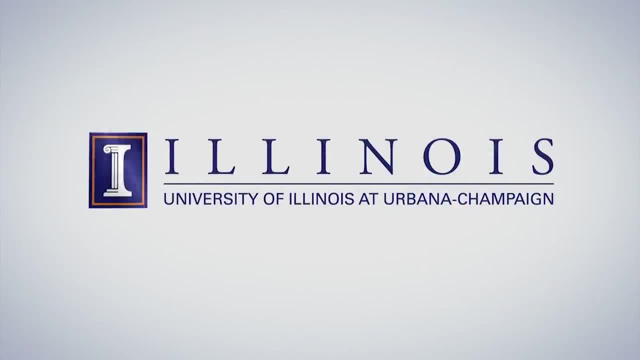 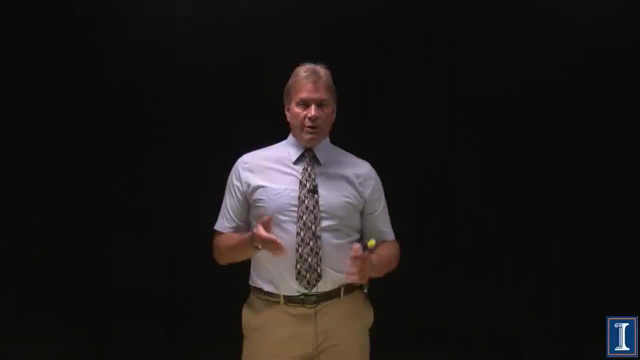 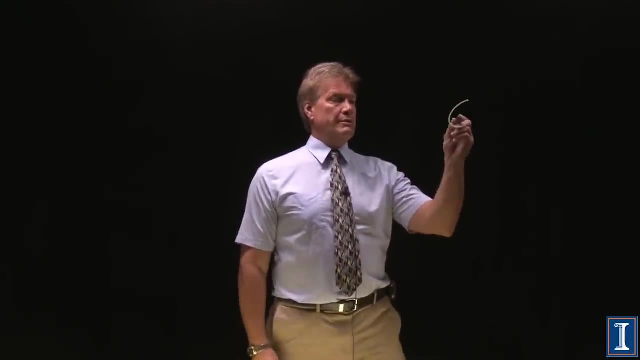 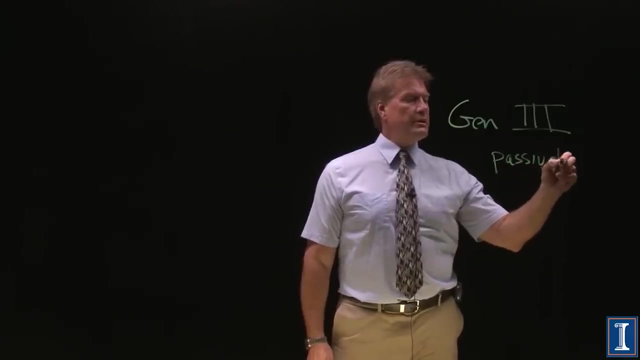 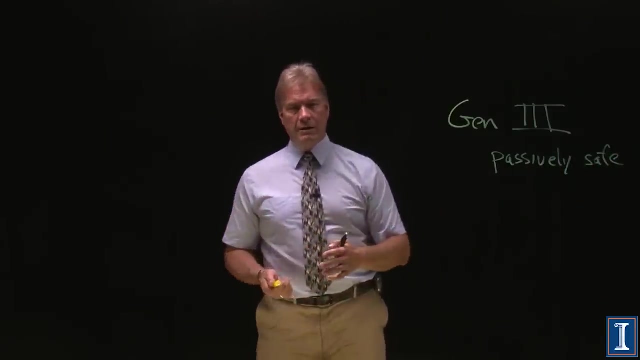 What's in the future for nuclear reactors? Today we have what are called Generation 3. Gen 3. And these have the wonderful feature of being passively safe. You don't need someone pressing a button, You don't need to keep the water on it, You can just use. 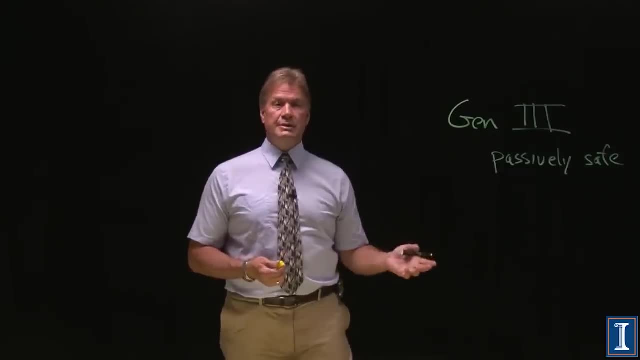 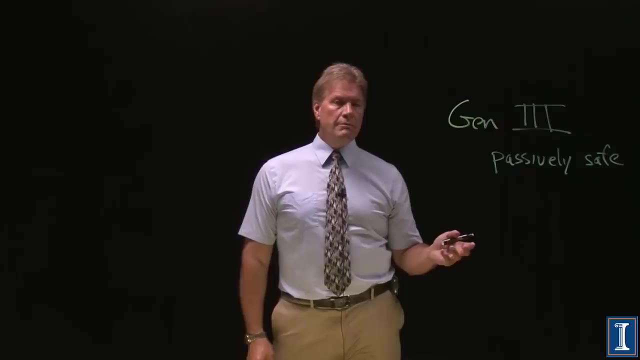 the laws of nature. convection to be able to take away waste heat in case everything goes wrong, And that's great. They have greatly improved safety. But other than that, they still have the same efficiencies. They still basically have the same types of design. 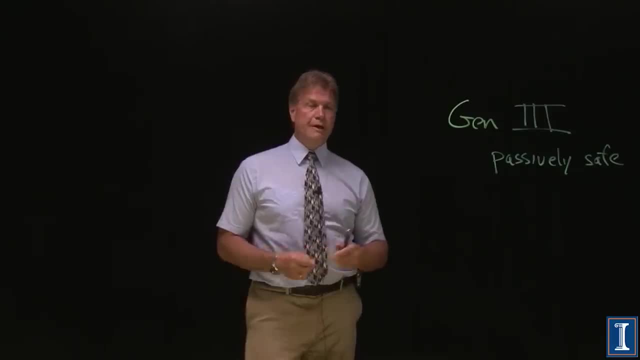 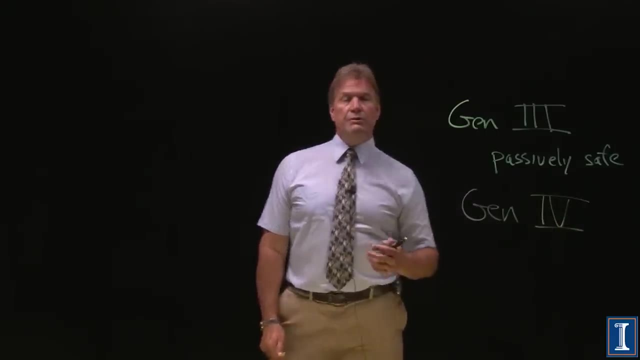 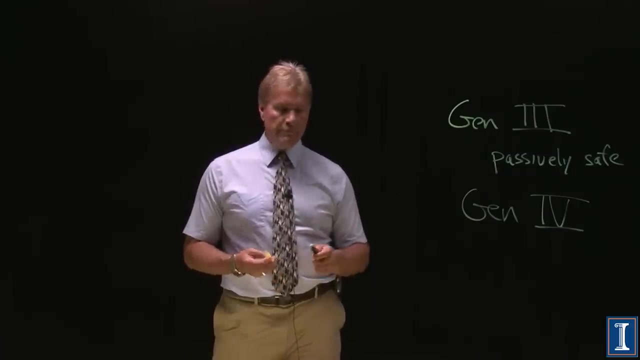 You're still fissioning uranium-235.. The future is called Generation 4.. And this is where you come up with the newer ideas to try to address some of the limitations from nuclear power. Safety is in pretty good shape, But these other limitations are usually. 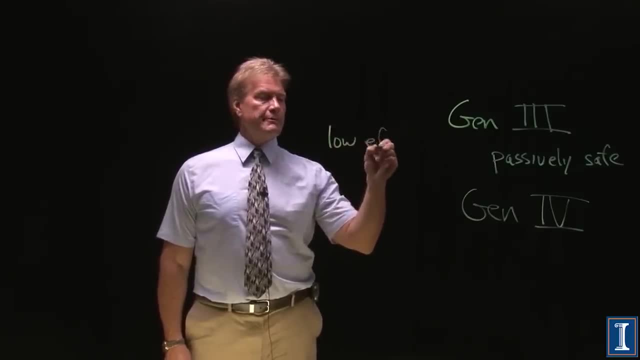 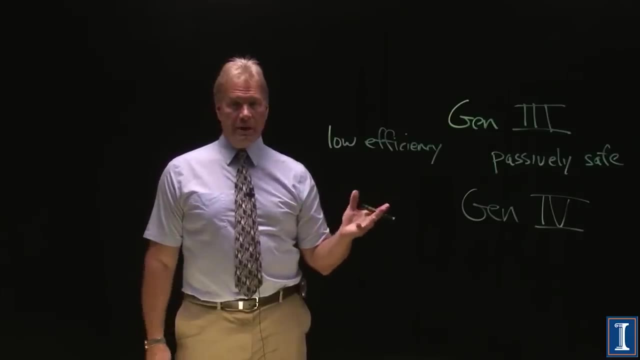 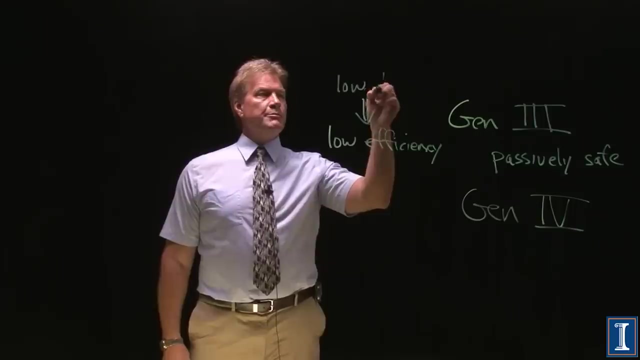 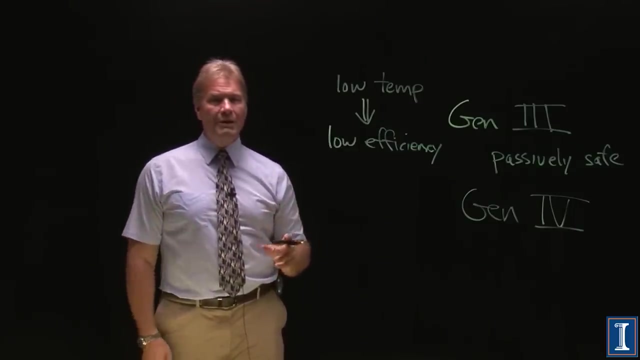 the low efficiency. Now, the low efficiency isn't all that low. It's about the same as coal plants or gas plants. This low efficiency is a result of having low temperature. You say, wait a minute. you're boiling water really hot under high pressure. That's certainly not low, Well relative. 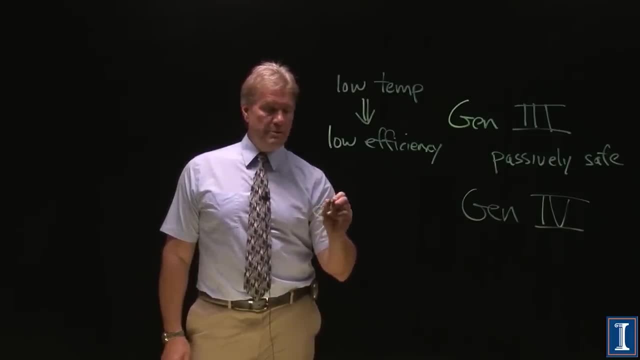 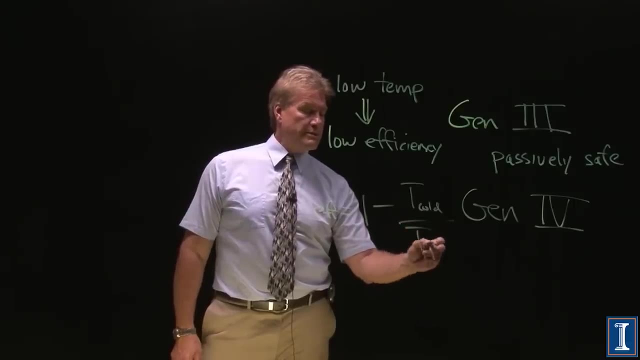 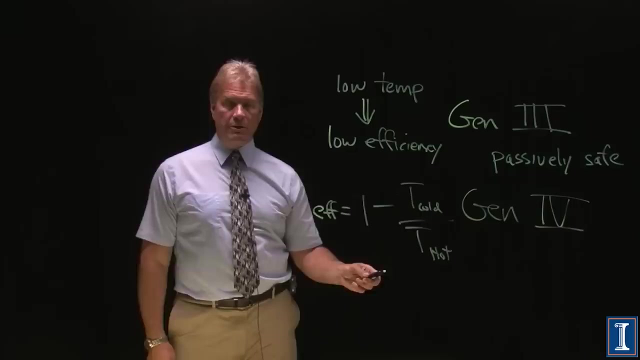 Carnot efficiency tells us that the maximum efficiency you'll ever get is 1 minus the cold temperature over the hot temperature. If I want this number to be closer to 1, I want this fraction to be near 0, cold I'm kind of stuck with. I've got the outside world. that's about as cold as you're going to get. 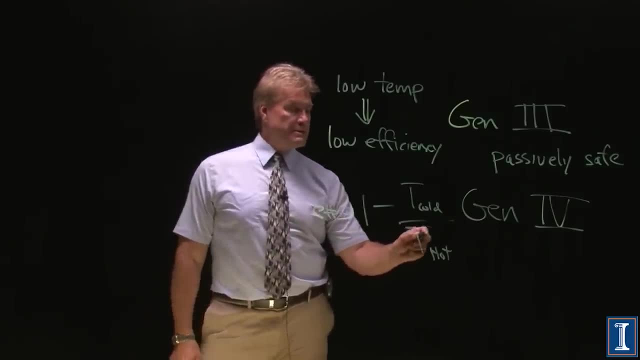 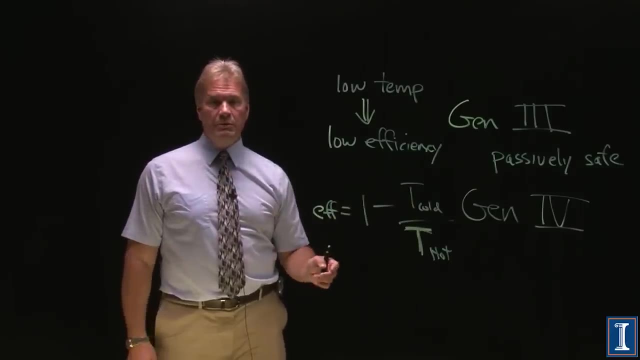 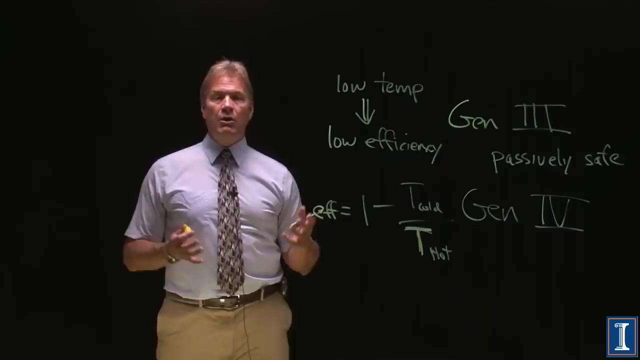 You're not going to spend electricity to refrigerate it. It means that I have to make this T-hot bigger. This would go to infinity. Efficiency would be 1.. So a desire in the new generation of reactors is to find ways to do this all at higher temperature. If you do it at higher temperature, you can do it in better efficiency And if you can solve other problems like downtime. reactors have to be refueled. It used to be. they would be shut for a month or two while you took out some of the old fuel and put in new fuel. Modern engineering techniques and attention to detail has improved that, and now many reactors are only shut for a couple weeks when they refuel every year. But another Gen 4 concept, besides going to higher temperatures, is to go to higher availability, Maybe something that's continuously fueled and therefore you never have some type of lack of ability of downtime. 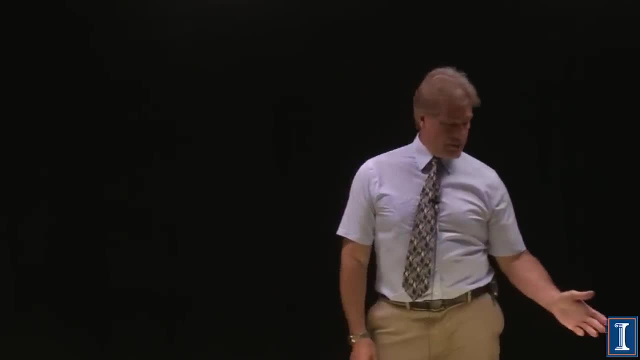 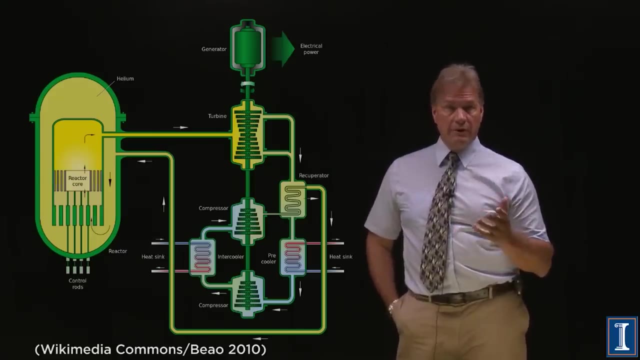 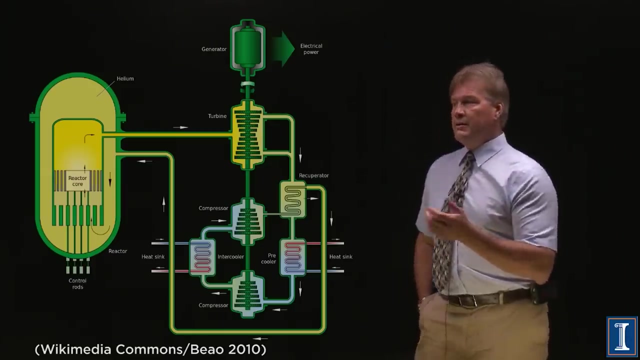 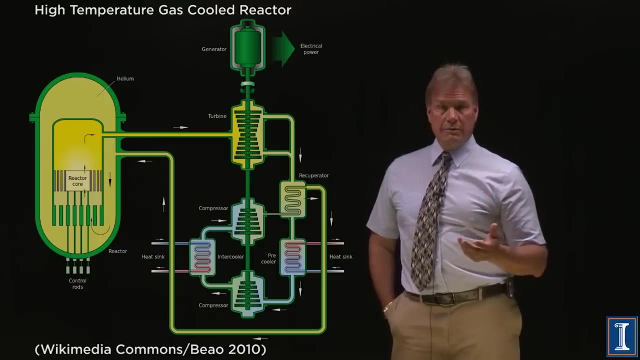 Let's look at some of these Generation 4 reactor concepts. Instead of using water- after all, it boils at 100 C- why don't we use something that's already boiling- A gas In the gas-cooled reactor? the high-temperature gas-cooled reactor. you don't use water. 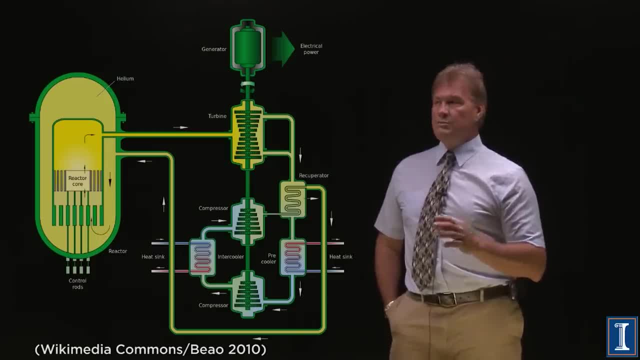 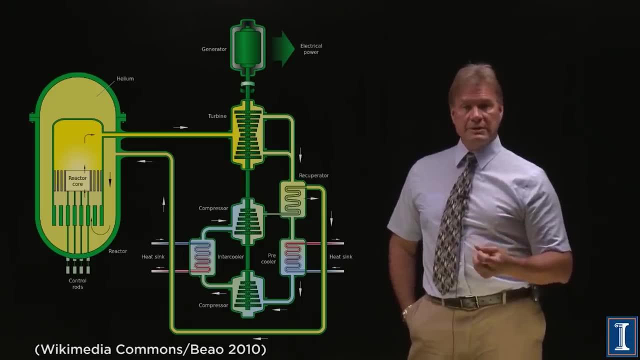 Now remember: if you're not using water, you need a different moderator. So in many of these cases they will use carbon or something as another moderator, But they can still be extremely safe because of their design. In the high-temperature gas-cooled reactor you use high-temperature gas. 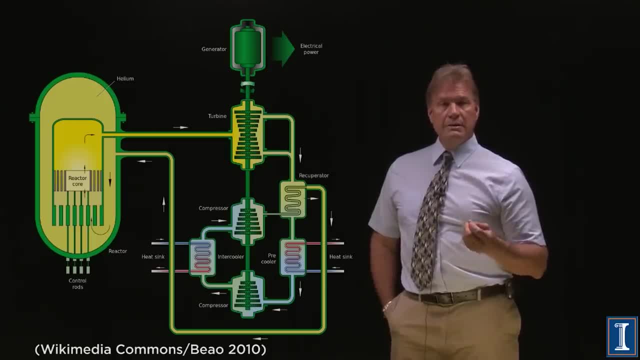 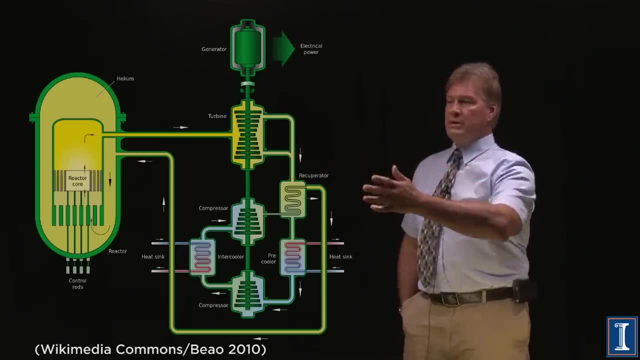 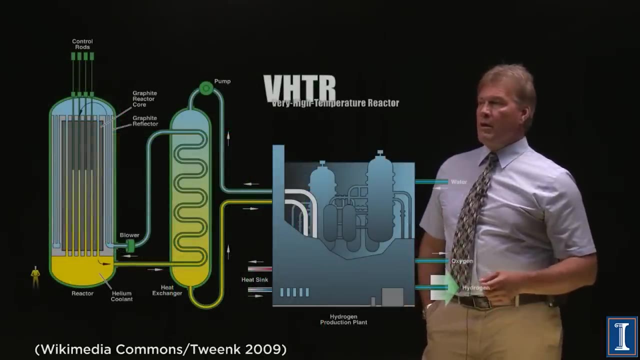 The fission products heat. It makes the gas even hotter And you can run it first through some type of gas turbine. The waste heat can then boil more water and go through a combined cycle. There's the helium-cooled reactor, the very high-temperature reactor. 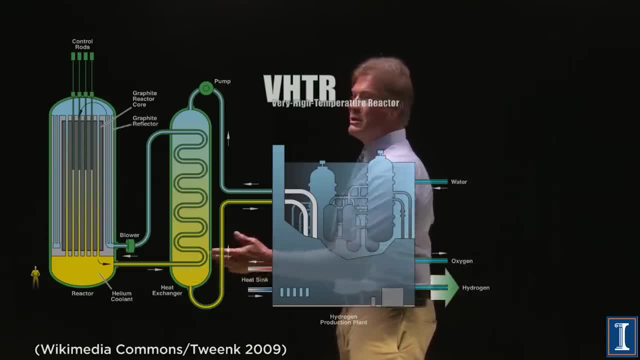 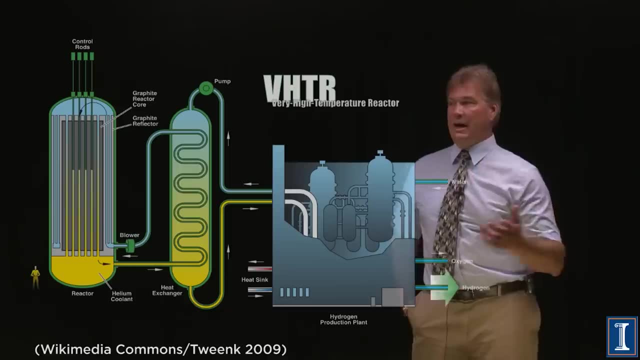 And likewise it uses a gaseous coolant, Since a gas is already a gas until you get it into its plasma state, which is ridiculously high, no solid material would even live to see that you can get things so hot that you might be able to just hydrolyze and take water and turn it into hydrogen. 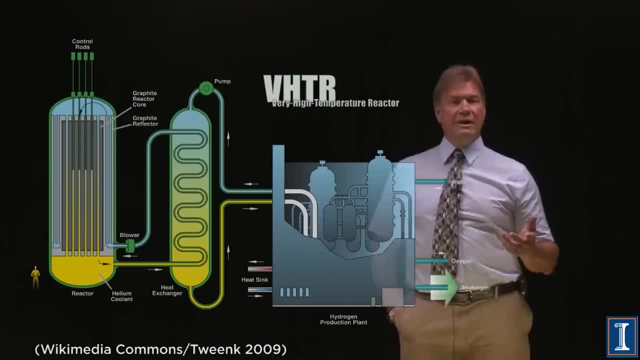 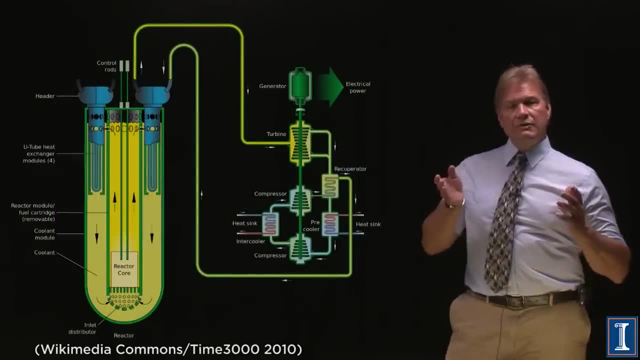 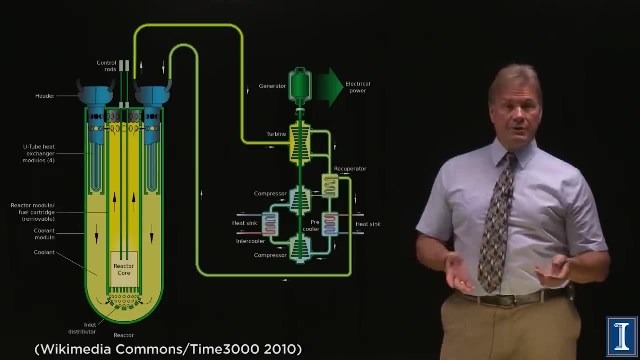 and not even have to go through a system of making steam to make electricity. This would be a wonderful hydrogen generator. Another scheme, instead of using water, is still to use a liquid, but to use liquid lead Sodder, for instance. 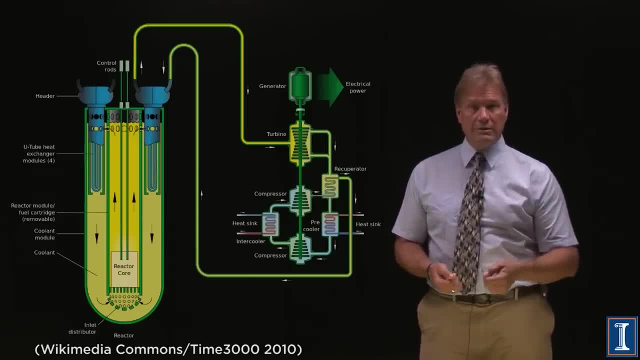 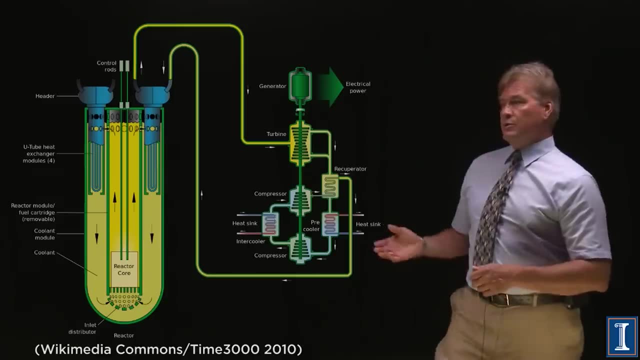 Sodder is often made of tin or lead or things like that, And you can melt it, A metal that melts at a relatively low temperature, but still a much, much higher temperature than water. So you actually move molten lead around and then do the same things you would do in a power plant. 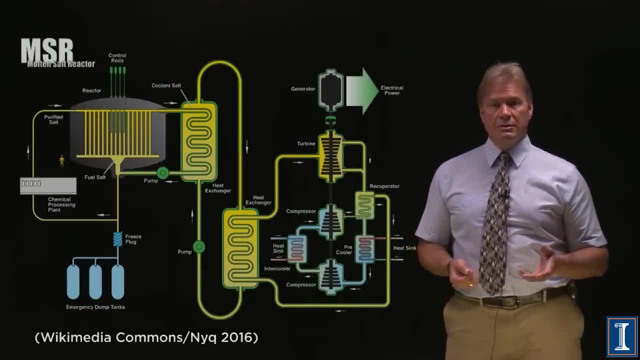 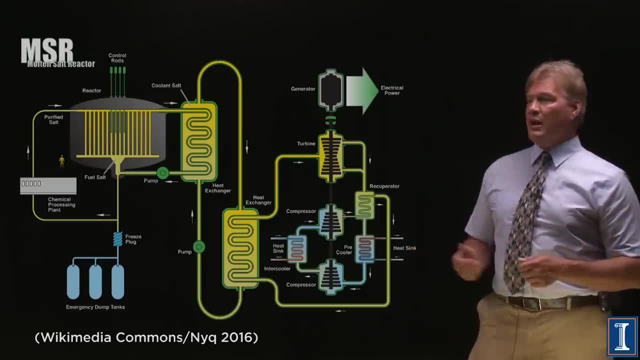 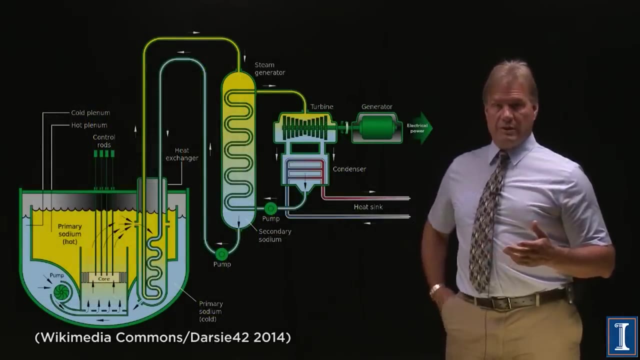 You could do it with sodium or some type of salt. You actually take salt, which we all think of as something you just eat, heat it up enough and it turns into a liquid And you use it as your cooling fluid. Or you can take another metal like sodium, a molten sodium reactor. 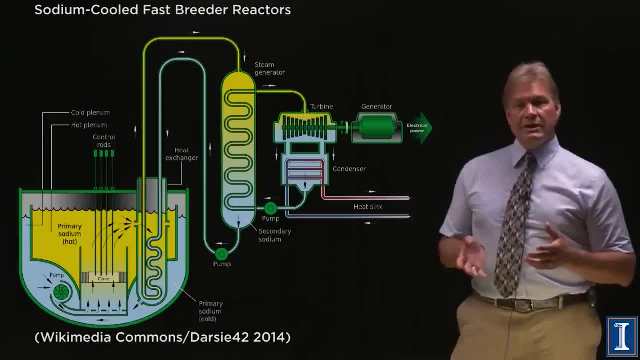 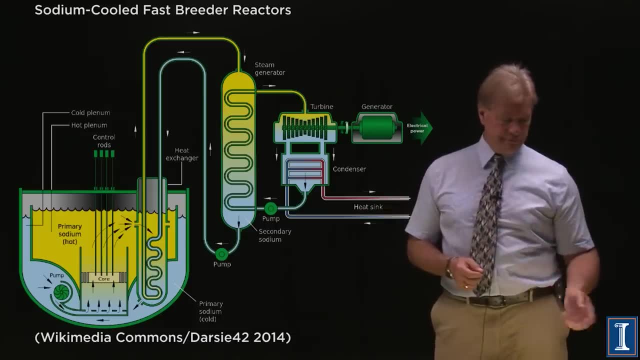 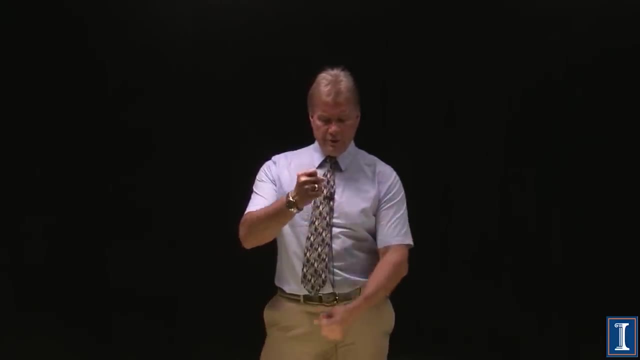 In fact this type of reactor has been used. The Phoenix and Super Phoenix commercial nuclear reactors in France were sodium-cooled fast breeder reactors. Now the things we saw before are still sort of your standard. I've got uranium in rods and I'm now just trying to run it all at a higher temperature. 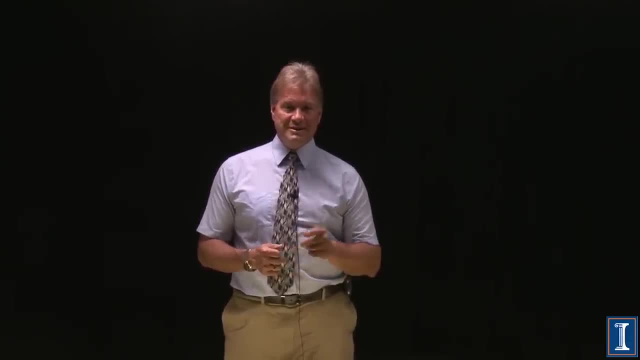 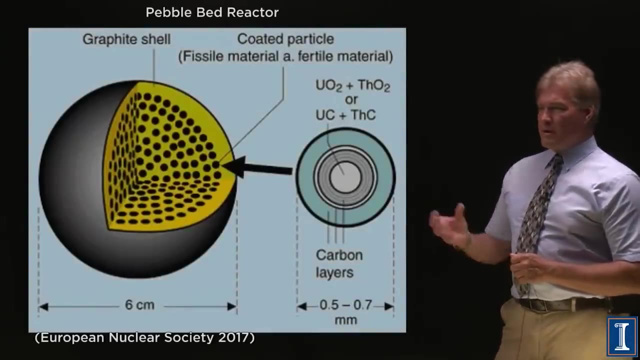 But Gen 4 includes a lot more stuff than that, Some things that are really, really clever, Like the pebble bed concept. So we're going to take these pebbles. you know almost a little less than baseball size, And inside you notice that there are a bunch of more smaller pebbles. 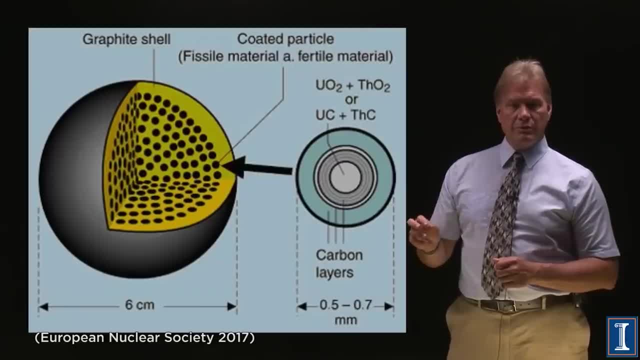 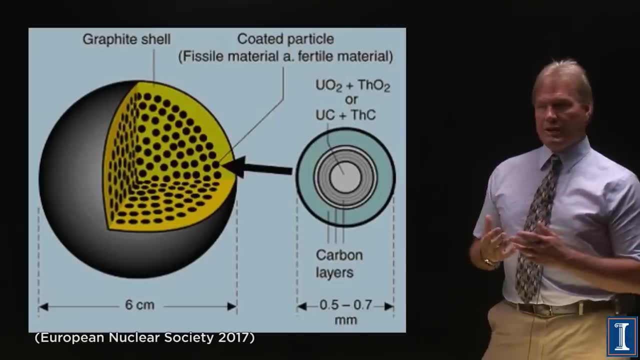 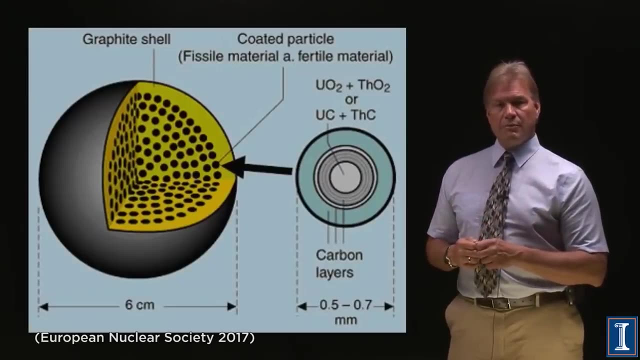 And those smaller pebbles have both the uranium fuel and the moderator mixed in, And this larger pellet here will allow fissions to take place, And it's made of very high temperature stuff. So as soon as fissions are taking place, this thing gets very, very warm. 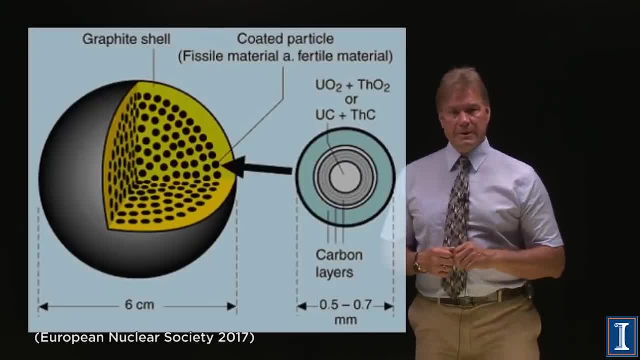 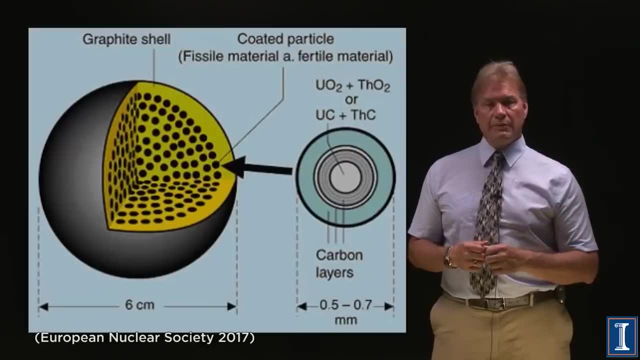 The pebble bed aims at two aspects. One is again a safety type of aspect And the second is a continuous refueling. You see, there isn't a lot of uranium in one of these pellets And if you design a system where it kind of works its way through a reactor, 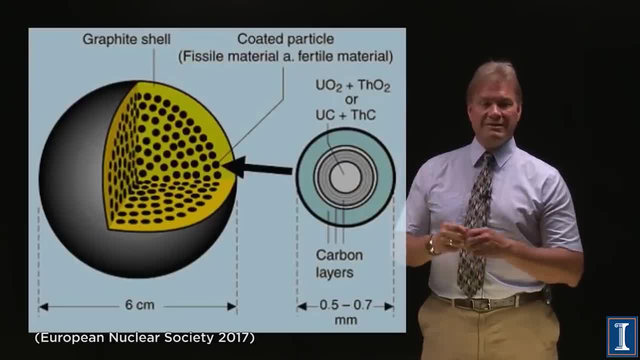 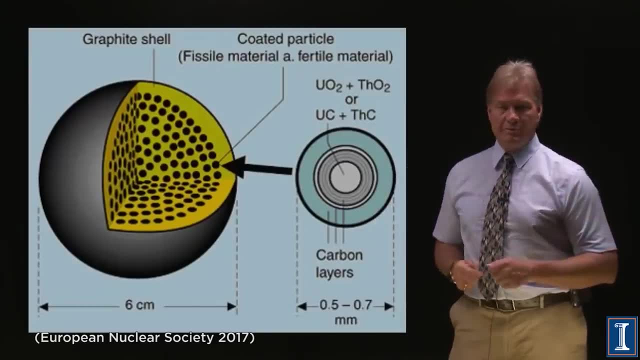 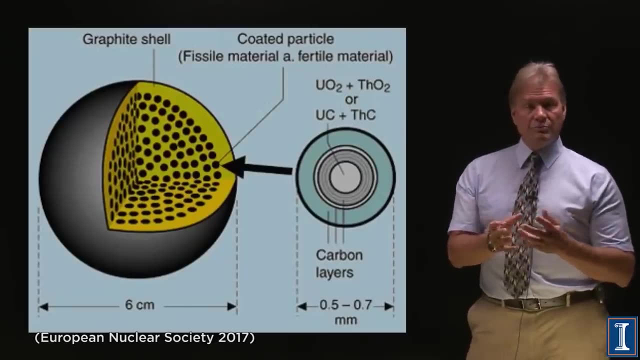 you can introduce new pellets in one spot and take out used ones from the bottom And maybe, if some of them get mixed up, you have a little testing to see how much uranium is left and then recycle them in. The other thing is if all these pellets fell down into a place where you had a neutron absorber, a control rod. 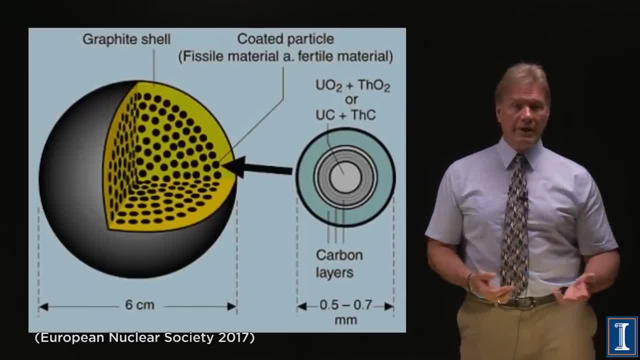 then of course there's no chain reaction. You've absorbed all the excess neutrons. no chain reaction takes place. To fluidize the bed, to have a fluidized pebble bed reactor, you would take this and put your coolant through it. It would push all the pellets up into an area where now there is no neutron absorber. In fact, there's an additional moderator of the coolant water And as long as that was there and you hadn't boiled all the water away, your reactor would operate great. 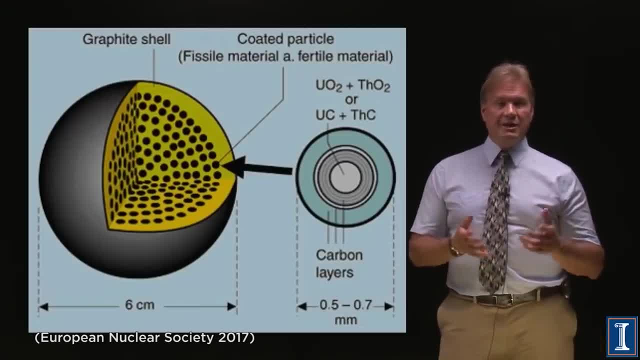 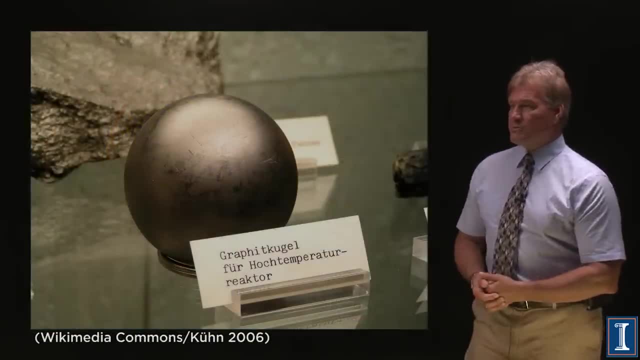 If it gets too hot and all the water turns to steam, guess what? all the pellets fall back down to where the neutron absorber is. Here's a picture of an actual pellet And you can see it's, compared to that note card, a little bit smaller than a baseball.